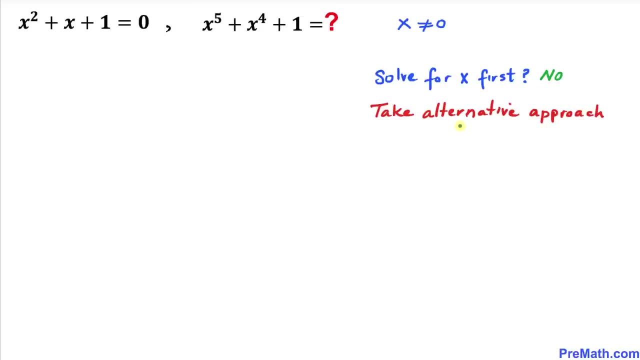 simple. So, therefore, we are going to take an alternative approach. So, therefore, we are going to think outside the box. So let's go ahead and manipulate our given these problems now. And here's our very first step. Let's focus on this very first equation, And here's- I have copied it down. Let's go ahead. 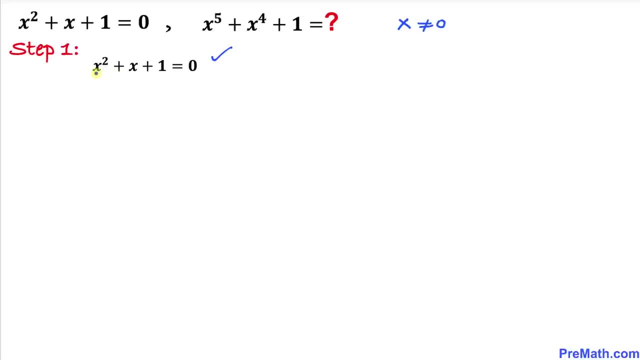 and manipulate this equation. Let's go ahead and divide by x across the board. I'm going to divide this side each and every time by x. Now let's go ahead and simplify: x squared divided by x is going to give us x plus x. divided by x is 1 plus 1. divided by x is equal to. 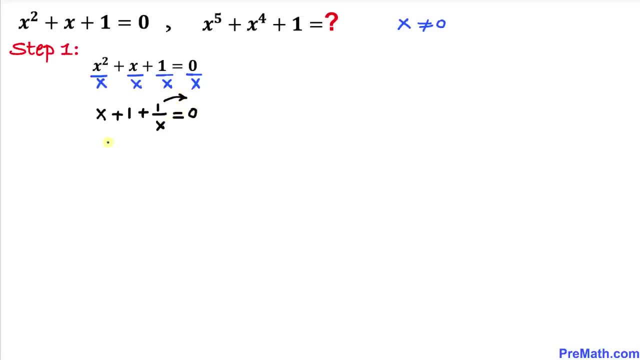 0. Let's go ahead and move this 1 over x on the other side. So we got x plus 1 equals to negative 1 over x. Let me call this equation as equation number 1.. And here's our next step. Let's focus. 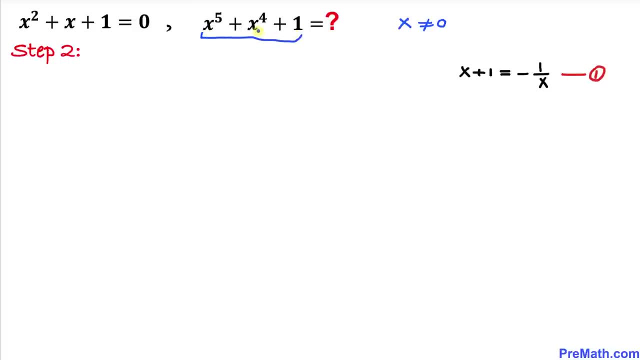 on this polynomial x power 5 plus x power 4 plus 1.. And here I have copied it down, And, as we can see, that x power 5 is equal to 0.. And here I have copied it down, And as we can see, that x power. 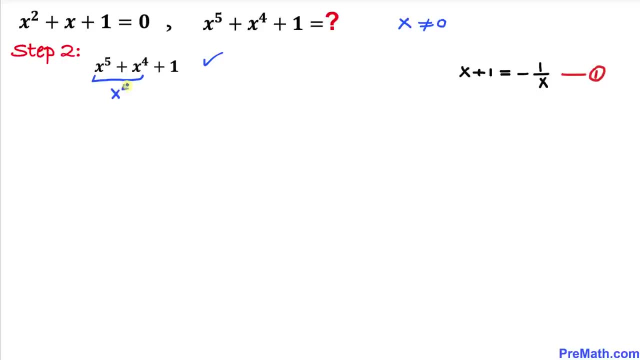 4 is in common between these first two terms. So therefore we are going to factor out x power 4 and inside parenthesis is going to be x plus 1 and then plus 1 outside, And now let's focus on this x plus 1.. We know from this equation: 1 x plus 1 is equal to negative 1 over x. So therefore I am: 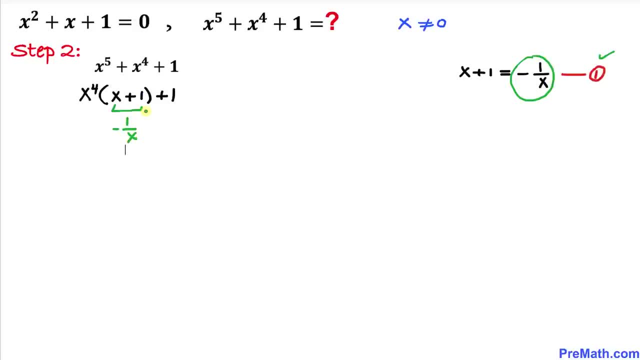 going to replace this one by negative 1 over x. And here I have copied it down. And here I have copied it down, And here I have copied it down. So let's go ahead and replace it. So x power 4 times negative 1 over x, and then plus 1.. So let's go ahead and simplify this thing. So x power 4. 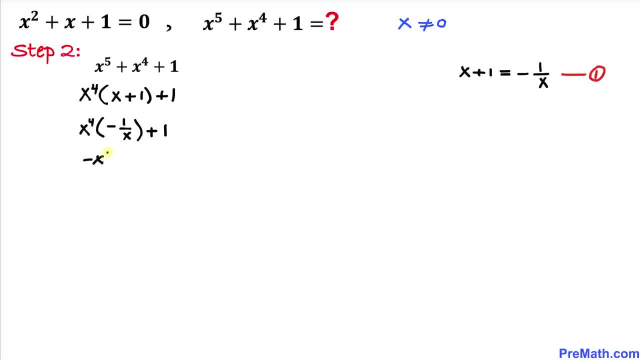 divided by x is going to give us negative x power, 3 plus 1.. Or if we switch it around, we can write this thing of 1 minus x cube. And now let's recall this famous identity: a cube minus b cube. and if I replace a by 1 and b by x, then we can write this 1 minus x cube as 1 minus x.